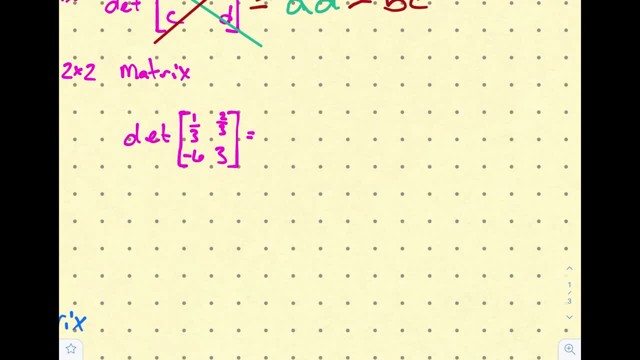 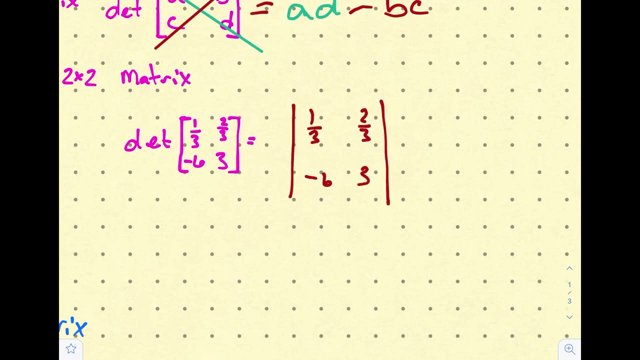 If I want to write the determinant of this matrix can also be written by the determinant of this matrix. So I'm going to write the determinant of this matrix as the matrix, but skipping the top and bottom that go on each bar. So this would signify the determinant of the matrix, which again is found by finding the difference of the diagonals. 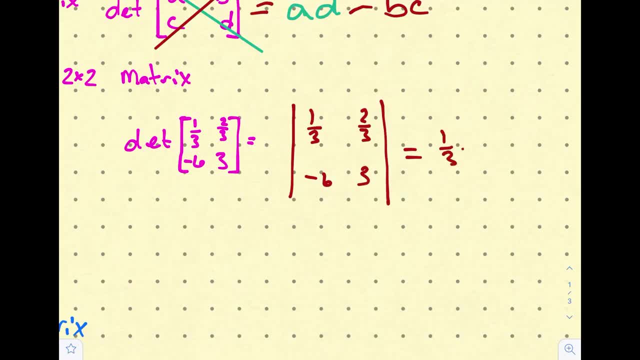 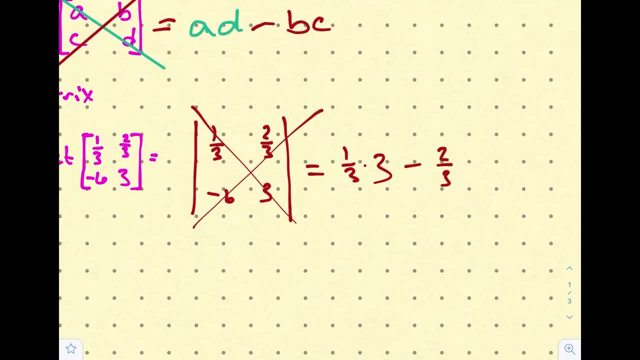 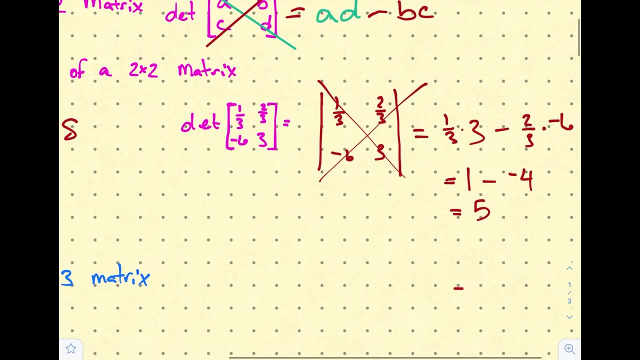 1 third times 3 minus 2 thirds times negative, 6.. 1 third of 3 is 1.. 2 thirds of negative, 6 is negative, 4.. 1 minus negative 4 is 5.. So the determinant of the matrix- 1 third, 2 thirds negative, 6, 3 is positive, 5.. 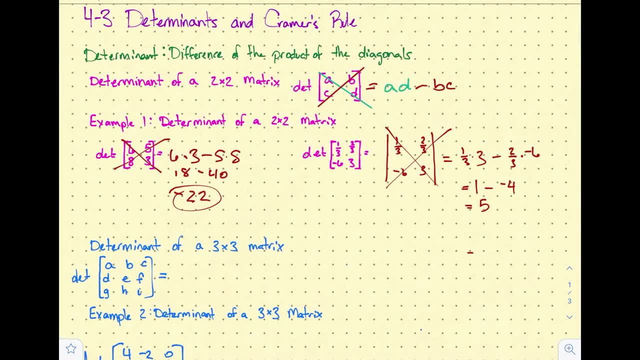 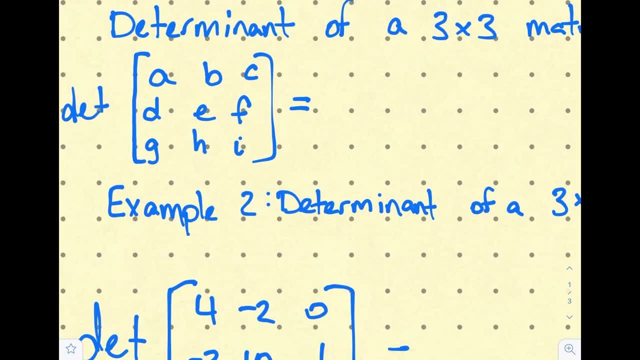 It gets a little more involved if we step up our square matrix to a 3 by 3. So we're going to find every diagonal going down to the right. So in this matrix, A, B, C, D, E, F, G, H, I. 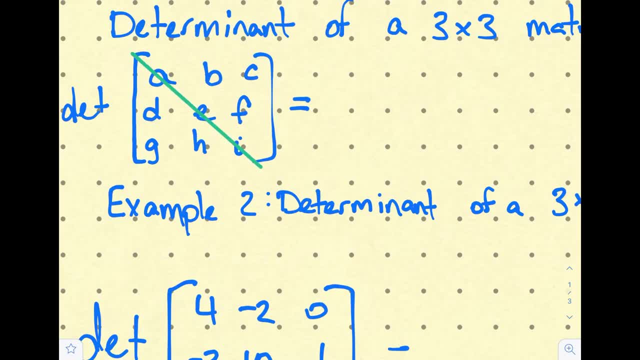 I will take my diagonals down to the right. So A E I. Then, as our diagonal runs out of order, we're going to find the diagonal that goes down to the right. So A E I. Then, as our diagonal runs out of room, we're going to carry it forward. 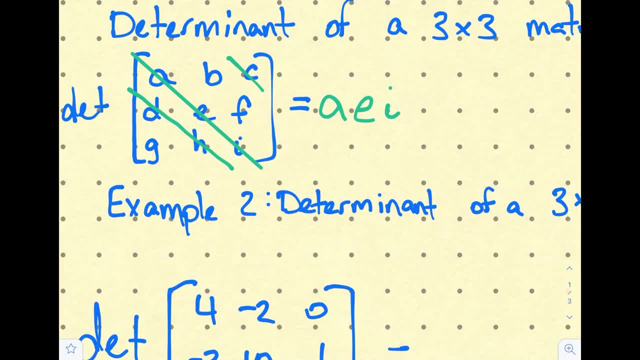 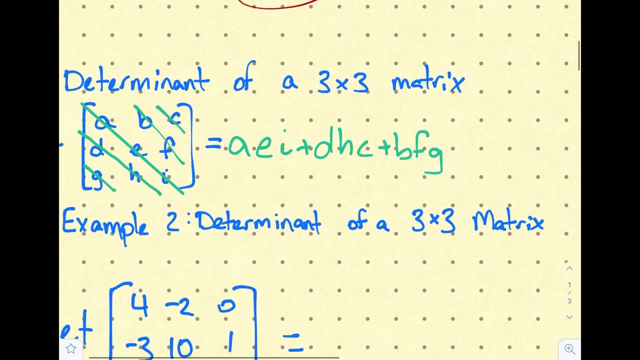 So D, H, C, And then the last three go together, B, F, G. So those are all the positive And we'll repeat the process going down and to the left, But those will be negative. So we have minus C, E, G. 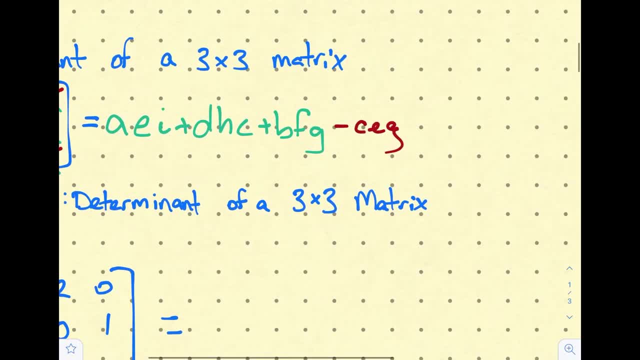 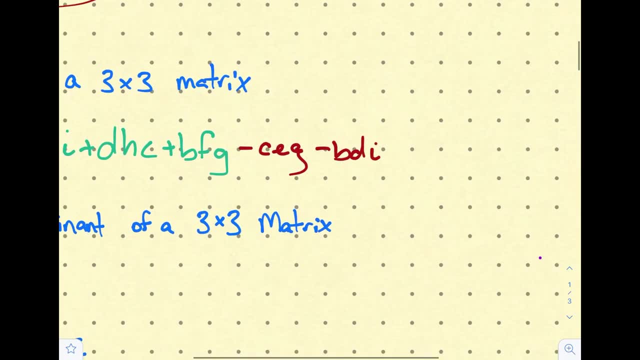 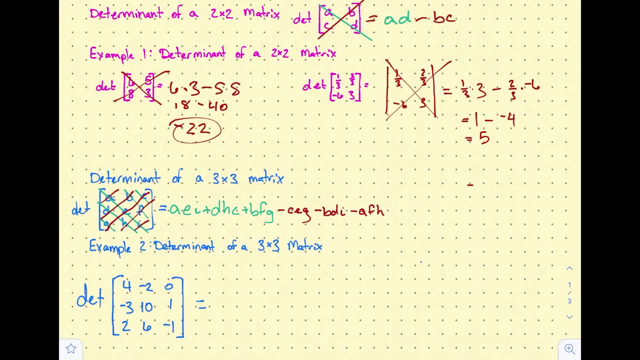 Minus B, D, I, Minus A, F, H. So the determinant of a 3 by 3 matrix is found using the same concept, Using the same ideas. It just gets a little more involved with our addition and subtraction. 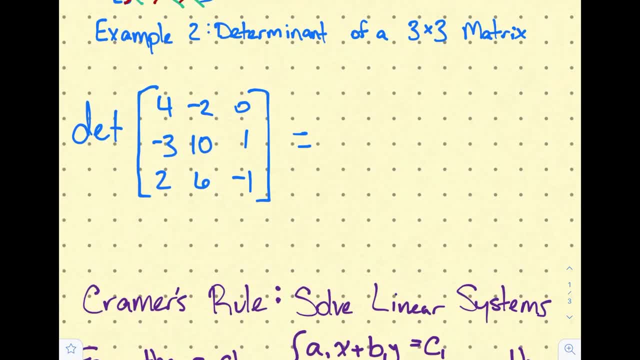 So let's find the determinant of this matrix, Which, again using our same kind of notation, we can rewrite the matrix But instead of using our normal brackets for the matrix, just use vertical bars. That signifies that I want to find the determinant of the matrix. 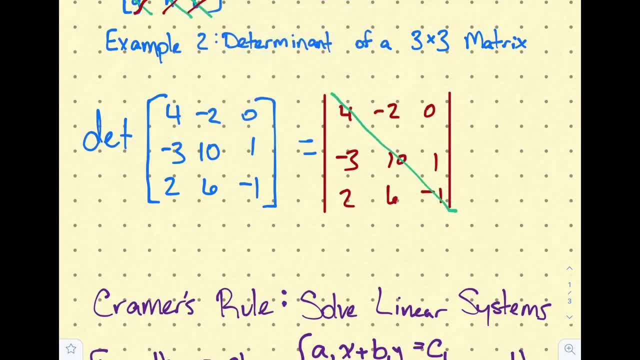 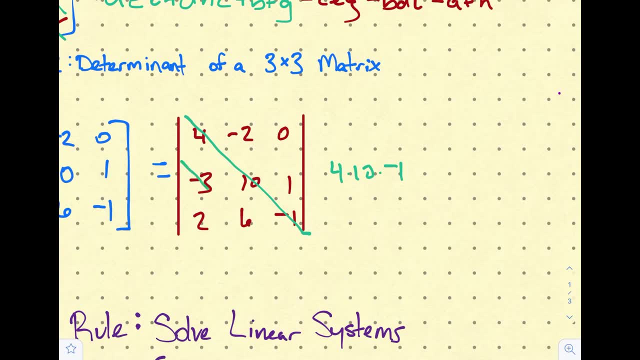 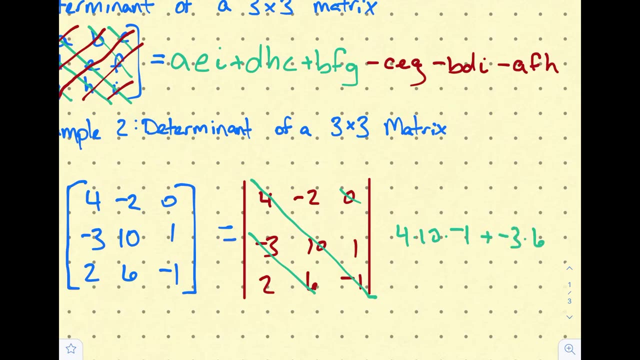 Which again will take our diagonals down to the right 4 times 10 times negative 1.. Our next one would be negative 3 times 6.. Negative 3 times 6 times 0.. And our next one is negative 2 times 1.. 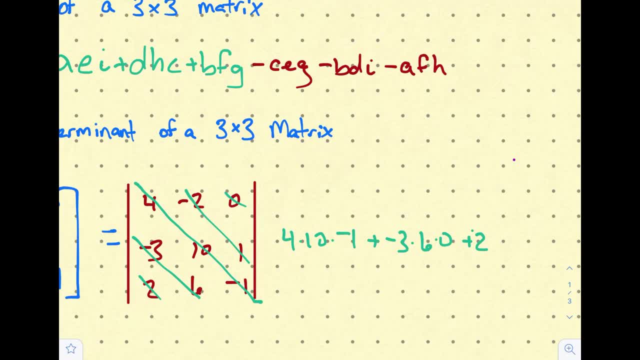 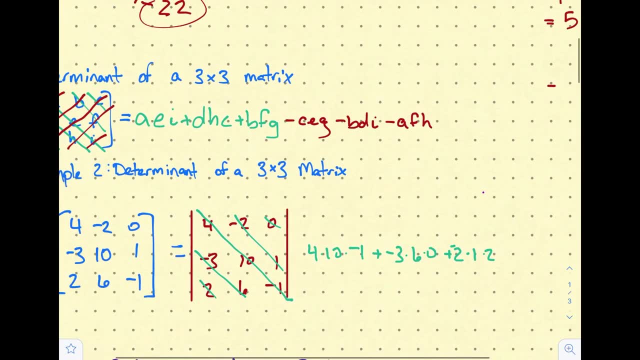 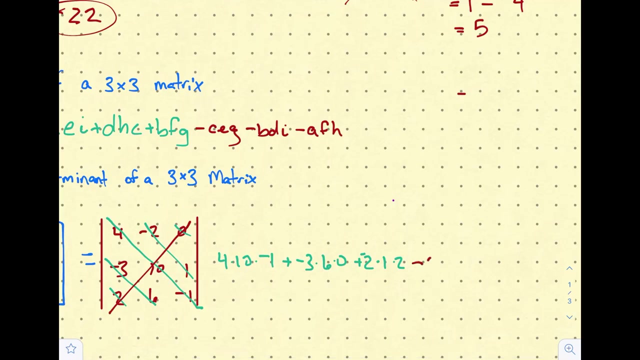 That's 2.. And then we will find all our matrices going down and to the, And then we will find all our matrices going down and to the left And subtract those. So minus 0 times 10 times 2.. 2 times negative, 3 times negative: 1.. 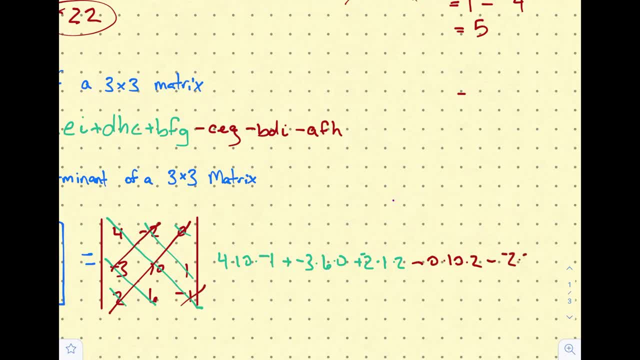 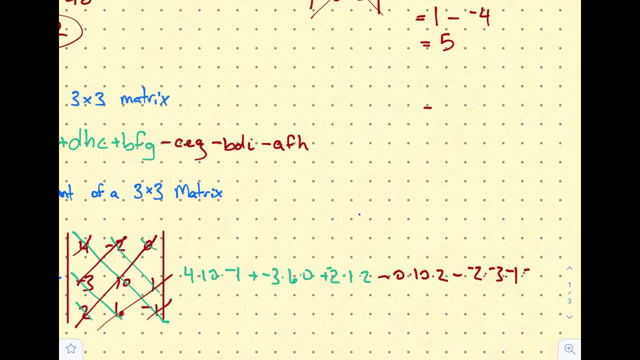 Sorry, negative 2 times negative, 3 times negative: 1.. And 4 times 1 times 6.. So let's find each product and then we will add and subtract as needed: 4 times 1.. 10 times negative: 1 is negative 40.. 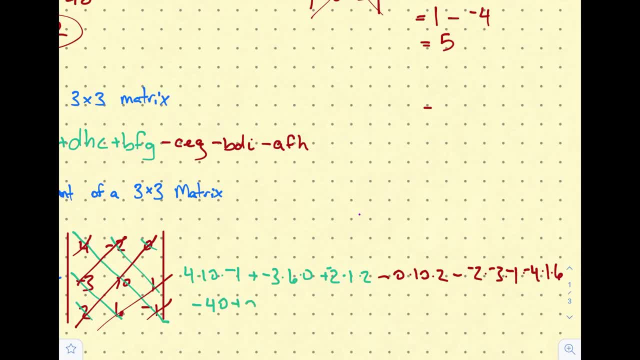 3 times 6 times 0 is 0.. Negative 2 times 1 times 2 is negative 4.. 0.. 0 times 10 times 2 is 0.. Negative 2 times negative. 3 times negative: 1 is negative 6.. 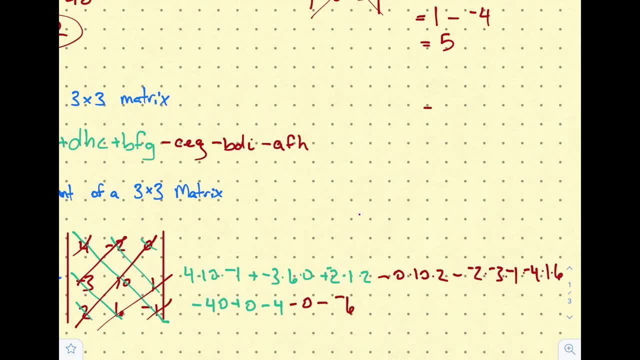 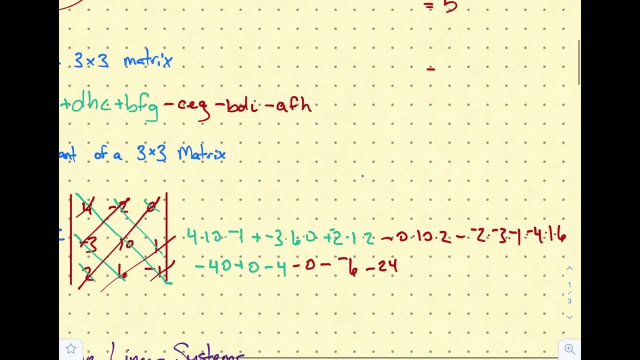 So we've got minus negative 6.. And 4 times 1 times 6 is 24.. Alright, negative 40 plus 0 is negative 40.. Negative 40 minus 4 is negative 44.. Minus 0 is still negative 44.. 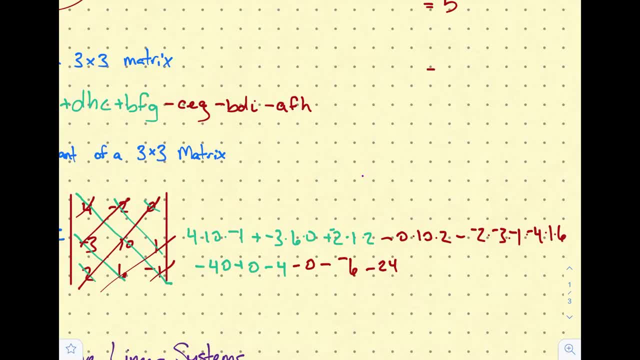 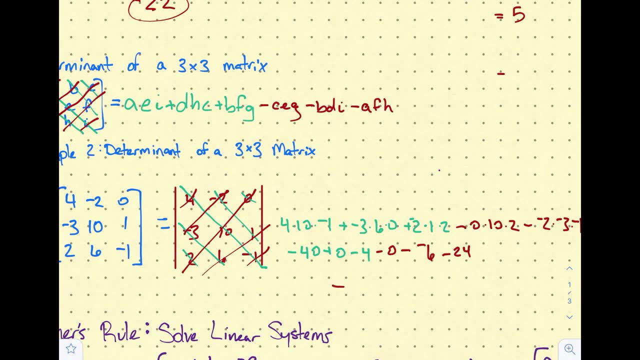 Plus 6, right minus and negative is plus is negative 38.. Negative 38 minus 24 is negative 62.. The determinant of the matrix: 4, negative 2, 0.. Negative 3, 10,, 1.. 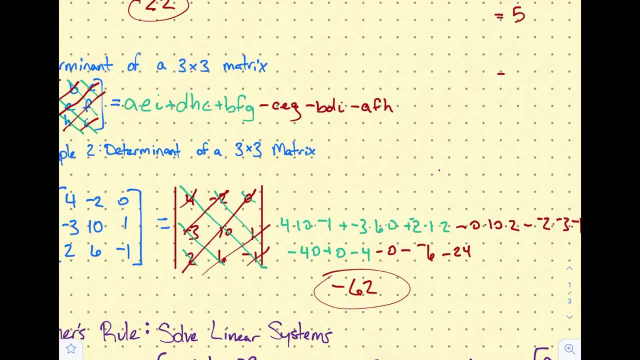 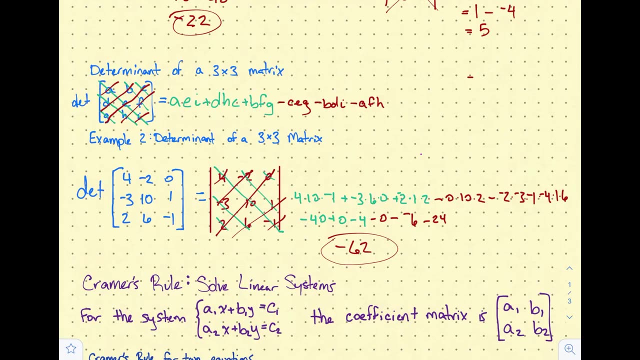 2, 6, negative 1 is negative 62.. Now there's a couple of different places that the determinant of a square matrix is useful. One such application is solving linear systems equations through what we call Cramer's Rule. So one important definition to have is if we have a linear system. 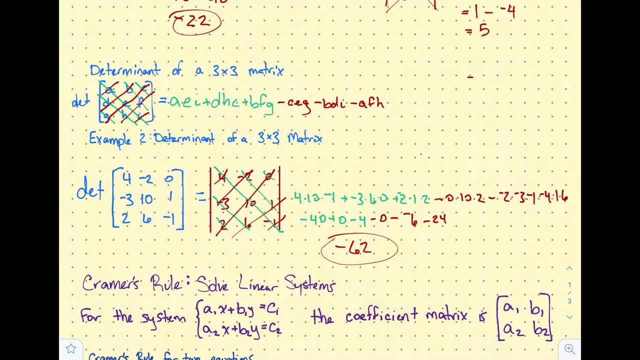 a1x plus b1y equals c1, and a2x plus b2y equals c2, we have what's called a coefficient matrix. This is just a matrix built on the coefficients of our x and y's, And we'll have an x column and a y column. 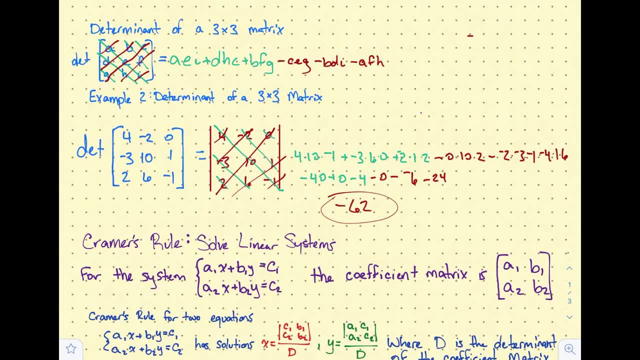 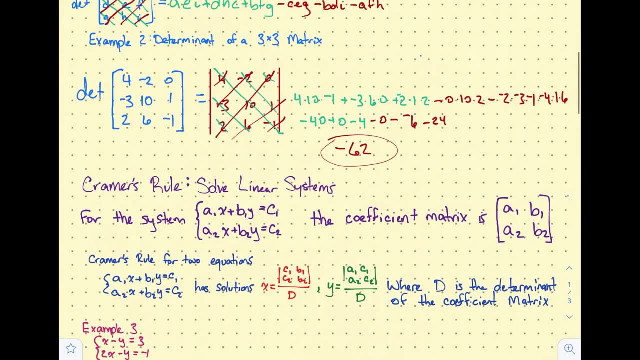 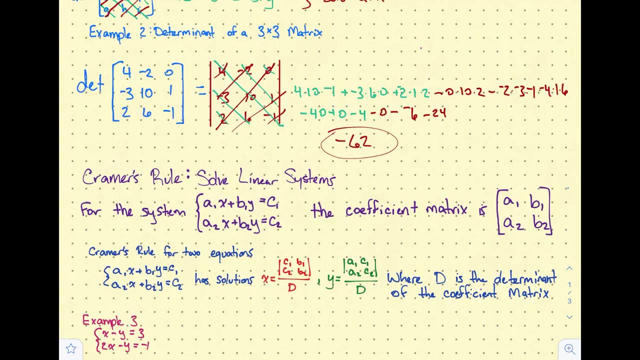 And one row represents the first equation and the second row represents the second equation. Cramer's Rule says that if we we can solve an equation, Cramer's Rule says we can solve a system of equations by swapping in the c terms for the variable we're looking for. 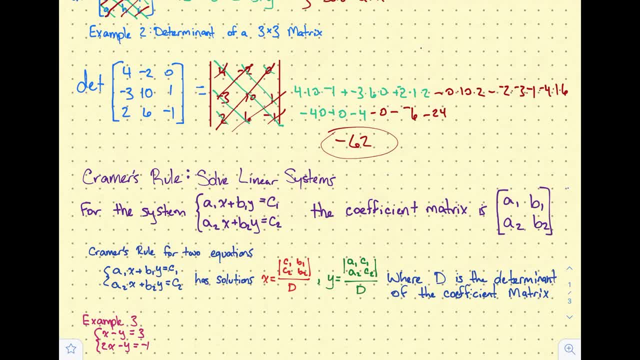 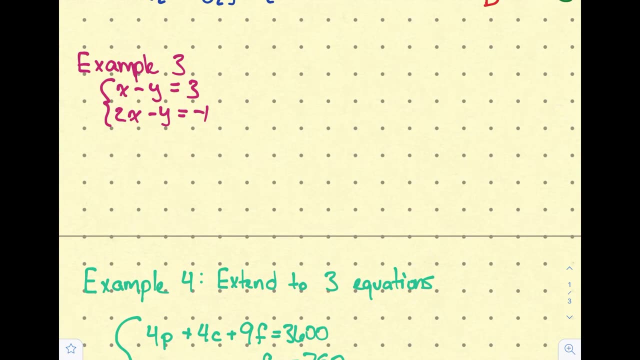 taking the determinant and dividing that by the determinant of the coefficient matrix. So let's do a couple of things. First I want to find my coefficient matrix. The coefficient matrix is 1 for my coefficient on x, negative, 1 for the coefficient on y. 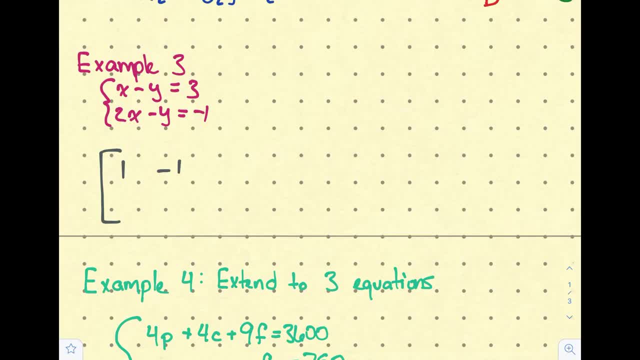 both from the first equation, 2 for the coefficient on x in the second equation, negative 1 for the coefficient on x, negative 1 for the coefficient on y in the second equation. So to solve both of for both x and y. 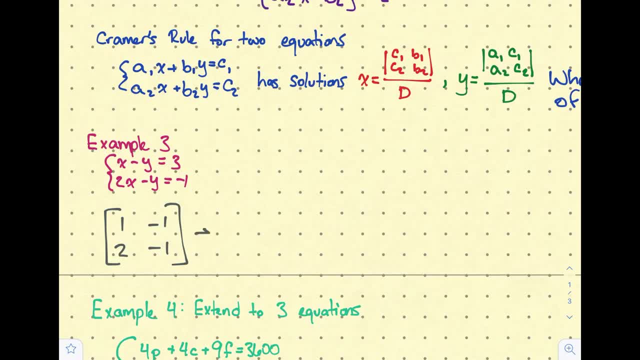 I will need to find the determinant of this. d is equal to the determinant, So that's going to be negative 1 minus negative 2, so the determinant is 1.. Plugging in our rule, it says that x is equal to. 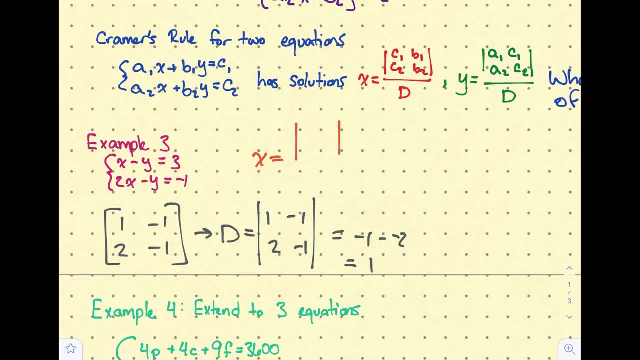 the determinant of swap in our c terms for the x's in our coefficient matrix, which was just these two numbers, and then divide by d, which is the determinant of our coefficient matrix. 1. The determinant of the matrix in our numerator. 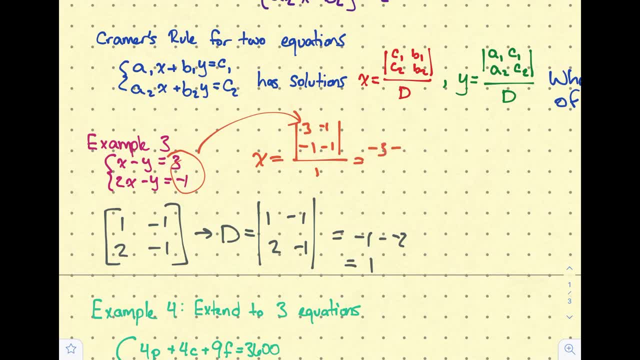 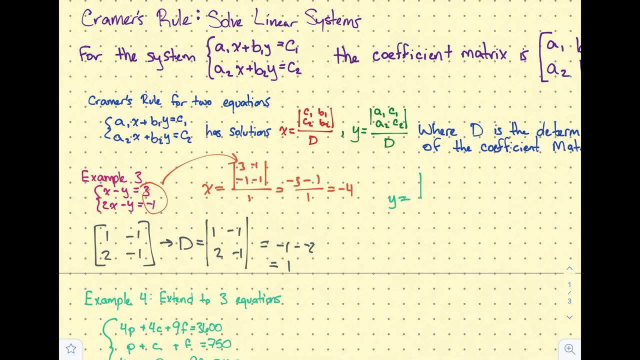 would be negative 3 minus 1, and then divide by 1, so we have x is negative 4.. And we can repeat this for y. Swap the c terms in for the y's in our coefficient matrix and divide that by the determinant of our coefficient matrix. 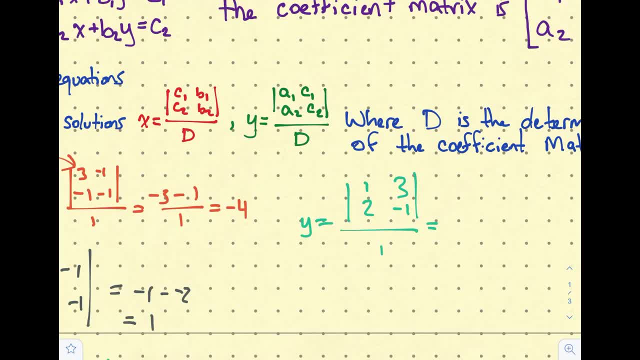 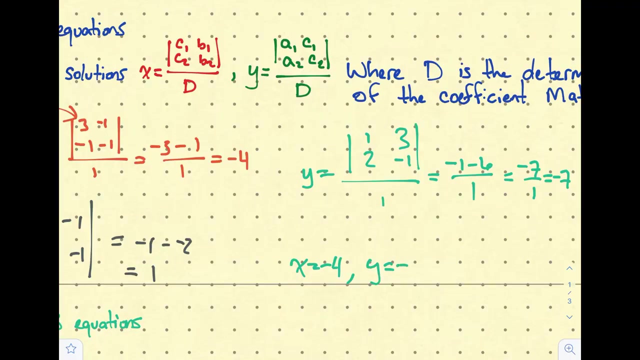 which was 1.. So the determinant of our matrix in the numerator is negative: 1 minus 6, divide that by 1, which is negative 7.. So the solution to this equation is: x equals negative 4, y equals negative 7.. 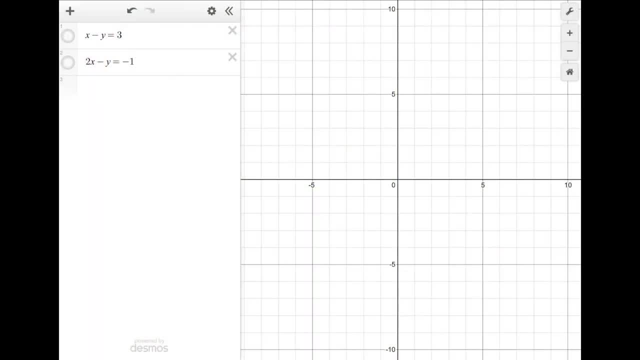 Now, one important fact to remember from studying algebra for all these years is that we can solve any equation by graphing. We can solve any system of equations by graphing. We just need to graph both equations and find where they intersect, And this is a good way to check our work. 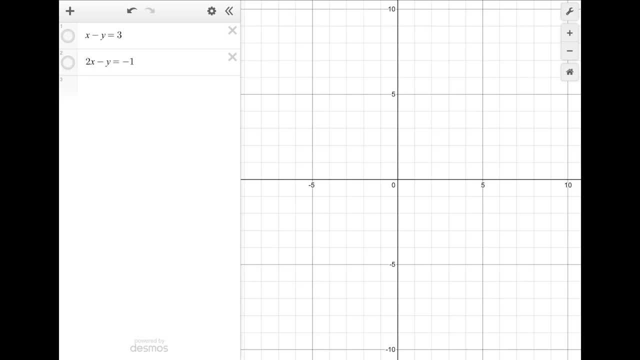 to make sure we did all our solving done correctly. So here I've got both equations: x minus y equals 3, and 2x minus 1, and 2x minus y equals negative 1.. So we'll graph each line. 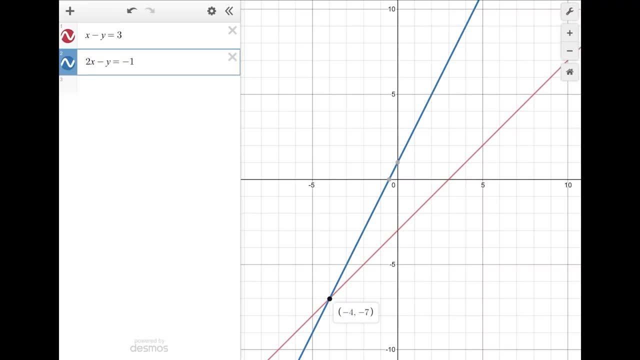 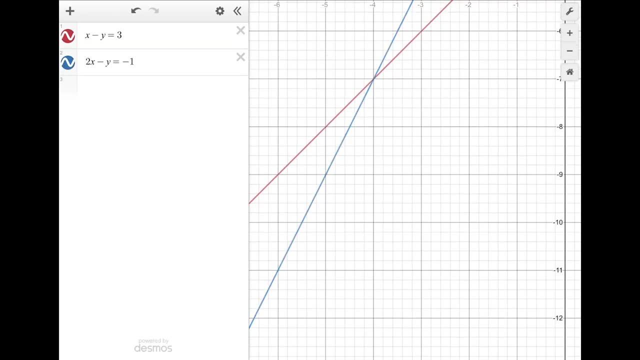 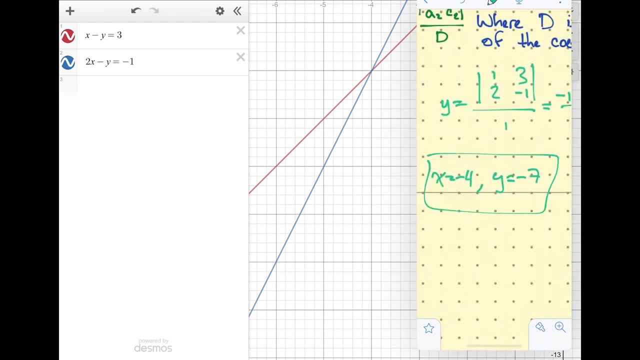 and find the point where they intersect. This point- negative 4, 7,- is our solution: x equals negative 4,, y equals negative 7,, which is exactly what we found when we solved this using Cramer's Rule. Thank you for watching. We'll see you next time.